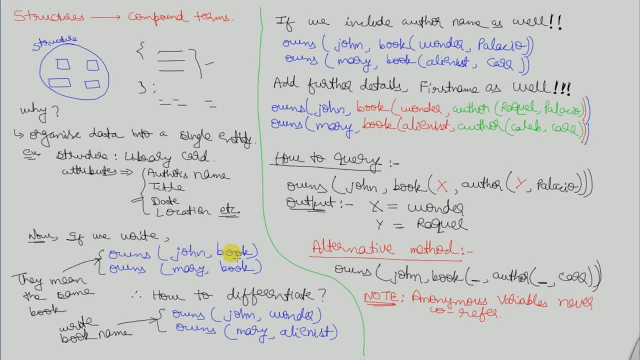 is a very simple structure and the first one means that john owns a book and mary owns a book. these two basically refer to the same book. so how can we differentiate? how can we differentiate that john and mary are owning different books? we can do it by giving the names to the book, like john owns. 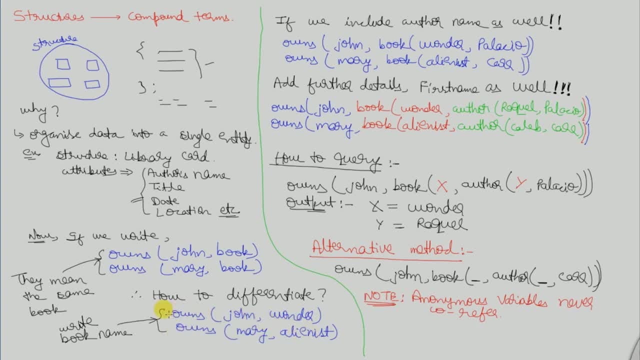 wonder and mary owns alienist. okay, so this is a very simple structure. let us look at nested structures. if we include author name as well, then how do we write it? we can write owns john comma book and then inside the book wonder palacio. that means john owns the book, which is 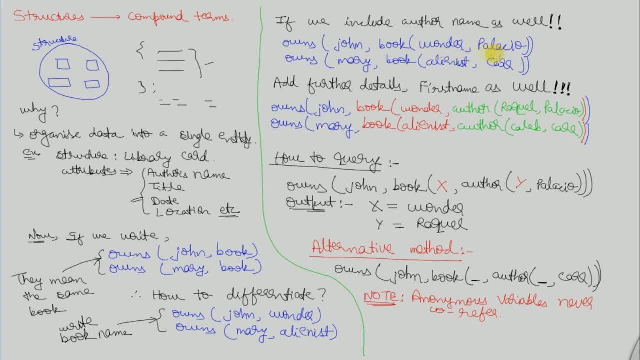 named as wonder and has been written by palacio. okay. similarly owns mary comma book alienist, comma, car. this means that mary owns the book alienist, written by car. these two are the surnames and these two are very famous books. you can check it out if you want. now, how can we add further details, like suppose, if there are? 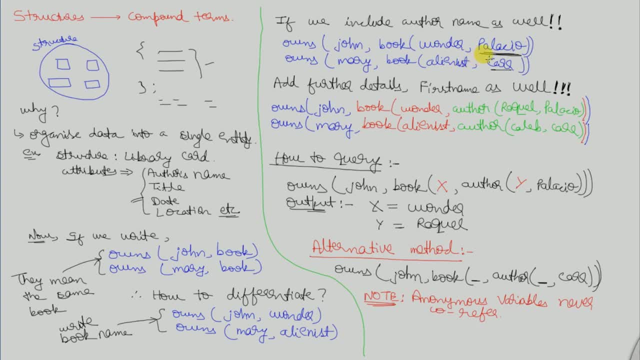 many writers with surname palacio. then how do we know that which palacio has written the book wonder? we can also add the first name as well. so how do we do it? we can even go further into the book master, so we will also have an example of the book master name being published. so how do you? 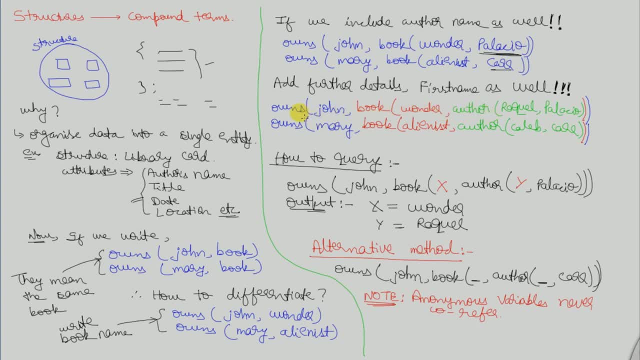 know that from the author's first name. you need a breakdown of the description of the book. so what does the book mean? so we can twisting this: Palacio, and similarly, Mary owns the book Alienist, which is written by Caleb Carr. okay, so this is about structures. now how do we query it if we have defined our?